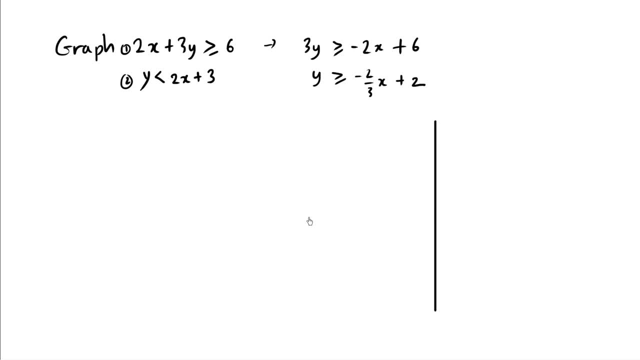 What does that mean? So if we have a nice graph, this is the slope. The coefficient of x is the slope. Negative slope means it's going downhill from left to right. This is the y-intercept. Positive 2 means we're going up 1, 2.. 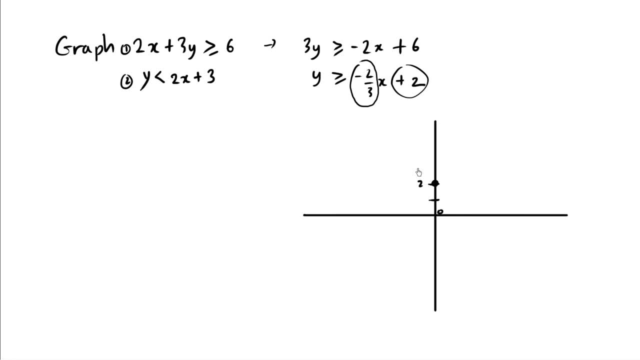 This is 2.. It's going to go through this point here. So a negative 1 slope is 45 degrees this way. So negative 2 thirds means it's a little bit steeper. So I'm just going to guesstimate around here. 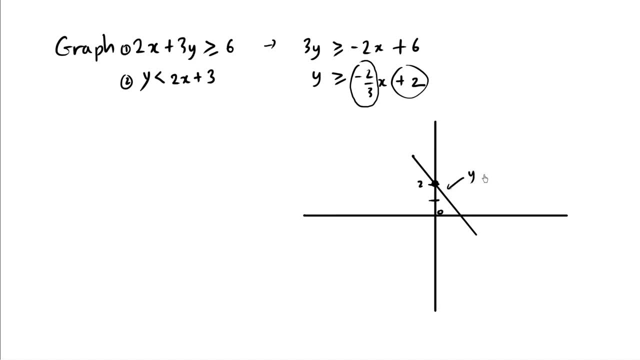 We're going to say that this here is the line. This is the line. y equals negative 2 thirds x plus 2. But for us we're thinking about the actual region that's above it. y is greater than means above it. 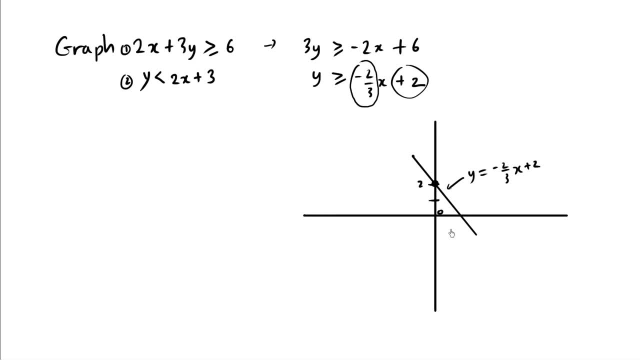 So when we're above it, we're going to shade in the possible solution region. The solution region is an actual area which extends onto infinity, So this whole yellow area is legit. Okay, so we have that as our boundary line And we have the greater than sign representing the actual area that's above this line. 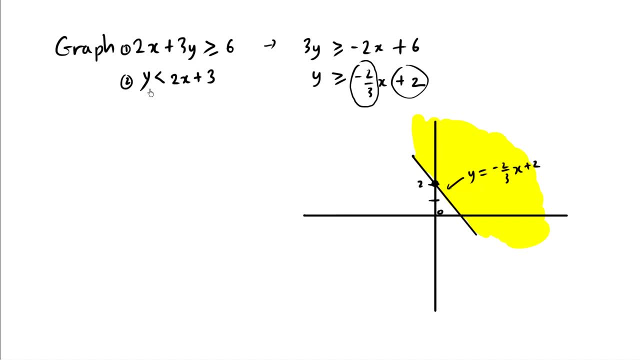 And let's try another line. now Let's try: y is less than 2x plus 3.. Fortunately this y is already isolated. So I know this is my slope And this here is my y-intercept. So y-intercept of positive 3 means it's definitely going to cross over here. 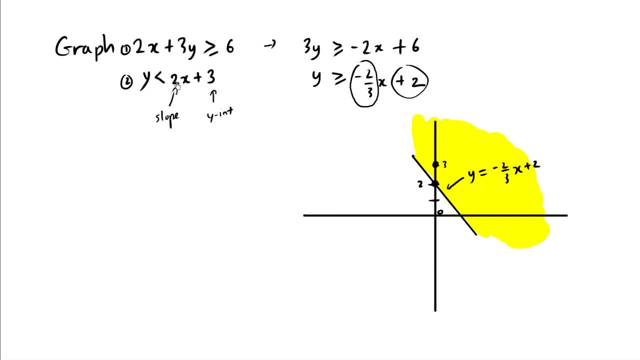 where the y value is 3.. And a slope of 2 means it's going to be. it's going to be steep left to right, It's going to go uphill. Slope of 1 is about 45 degrees. The slope of 2 is a little bit more steep. 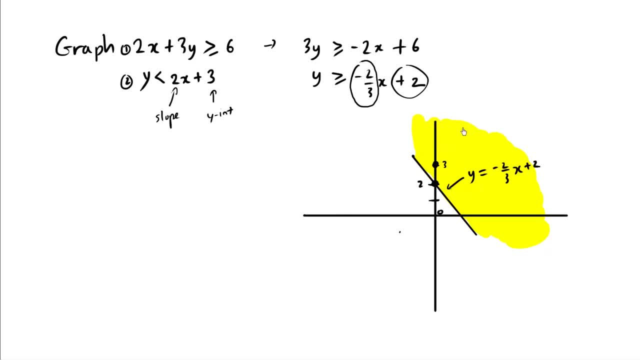 So let me just try guessing around here. Let me just try that again Around here. Now this one here I'm going to actually make it dashed, So I'm making this line a little bit dashed. The reason why this line is dashed is because we have a less than sign. 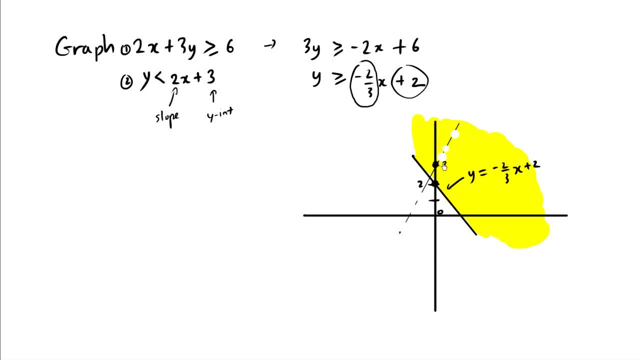 not a less than or equal to sign. So we don't actually include the solutions actually on the line. So when we say that y is less than, we're only looking at the actual values. that's below it, So we're looking at the values over here.